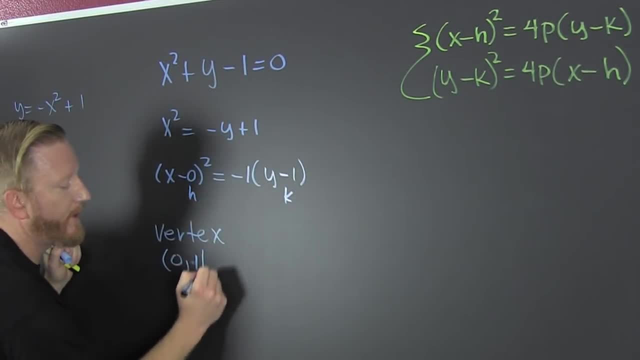 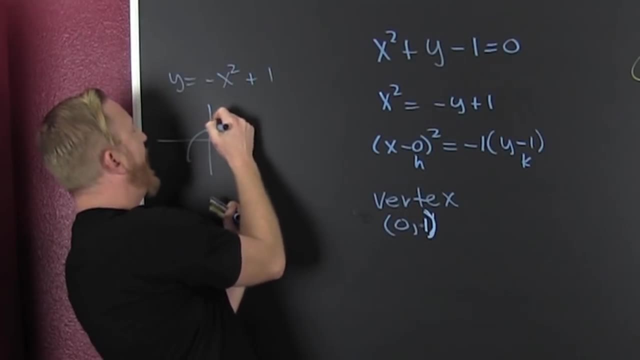 in there. zero one fun. get over there. curves, accentuate your curves. your vertex is the point which point, this point? oh, look at that, all right. so I need to also find my focus and my. 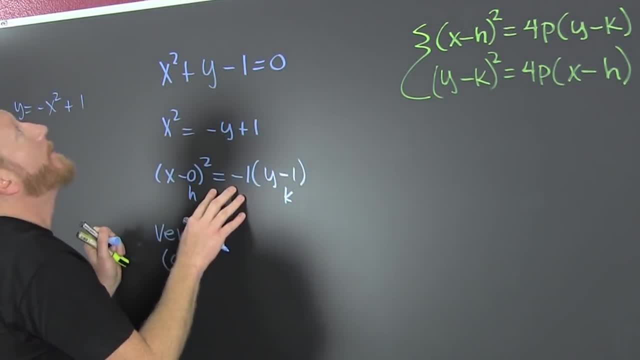 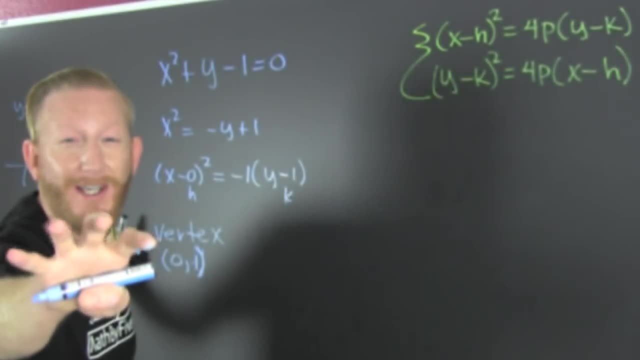 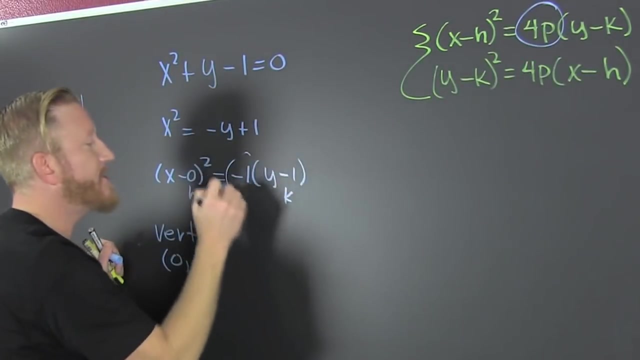 directrix, because the parabola is defined to be the curve equal distance from a point in the line. the point is called the focus, focus, people focus and the line is called the directrix. so first we need to find our p. in order to find our p, we're going to match these guys up. 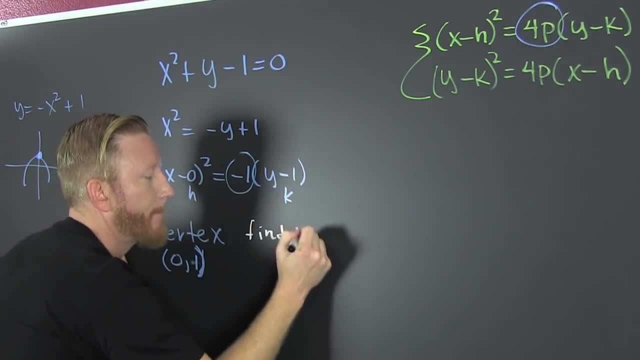 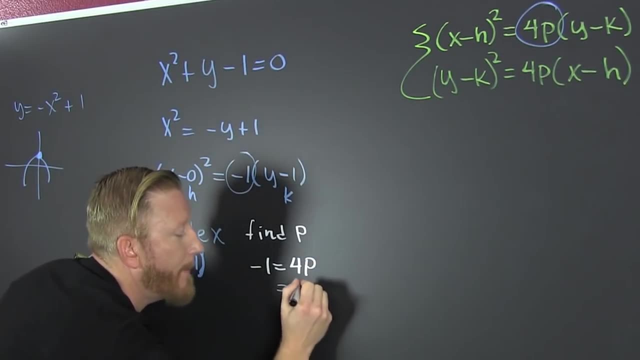 so find p, find p, all right. so then minus one is equal to a four p. so it turns out to me that my p is a minus 1 fourth. Now, what's that? That's the distance away from the focus that the 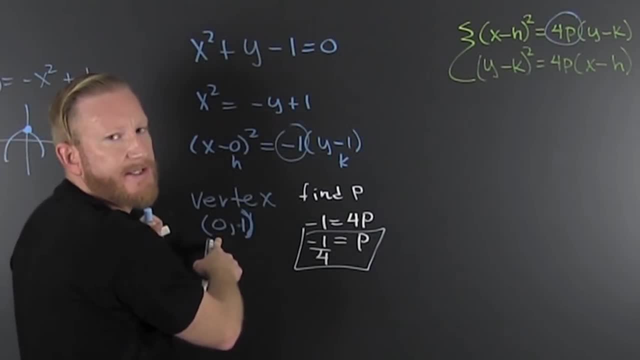 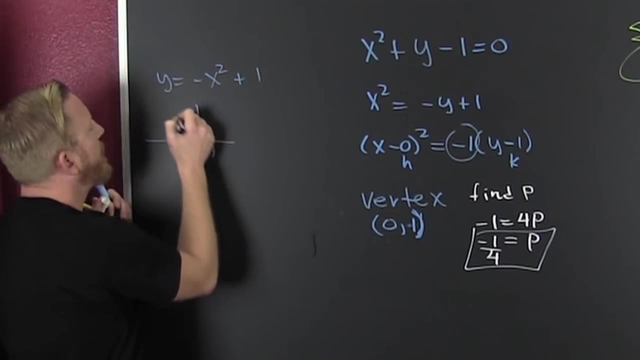 directrix. that's the distance away from the vertex that the focus and the directrix lie. So I'm looking at this and what am I changing? I'm changing my y. Yeah, So that means I need to change that y. So if I'm finding the focus, is the focus. 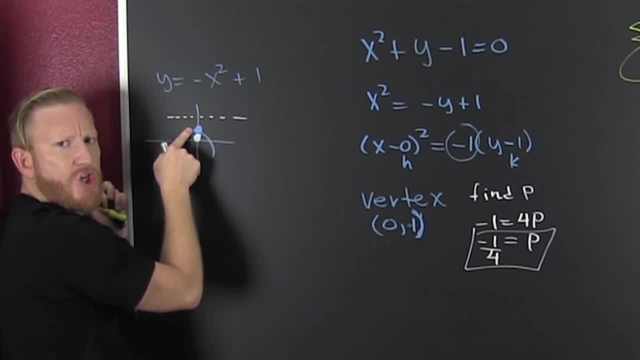 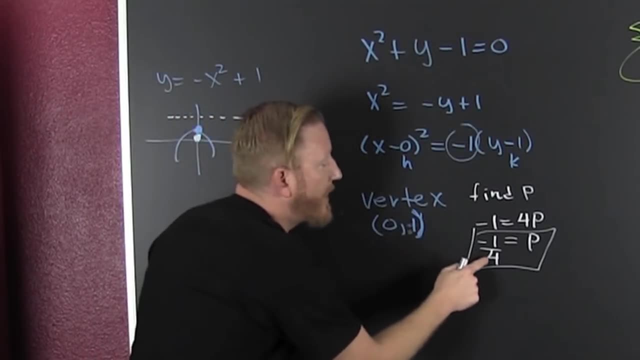 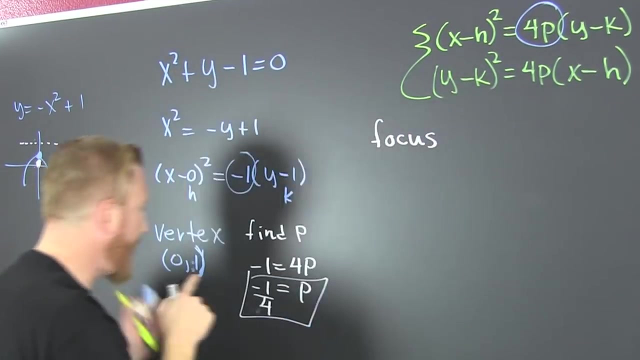 bigger than or smaller than. Look at it, Look at it, Look at it, The focus is smaller than the vertex. So I'm going to take that y value and I'm going to subtract off 1. fourth, Yeah, So focus, I'm going to take that y value, y because I'm changing my y, All right, So 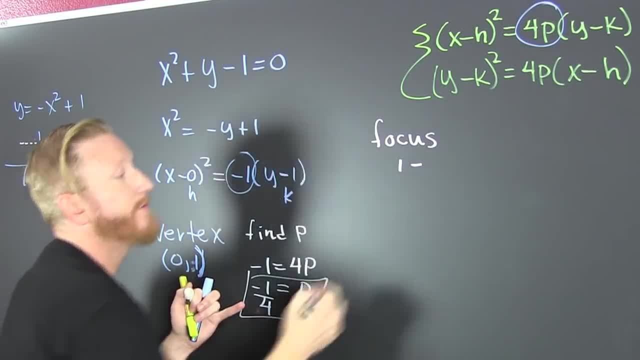 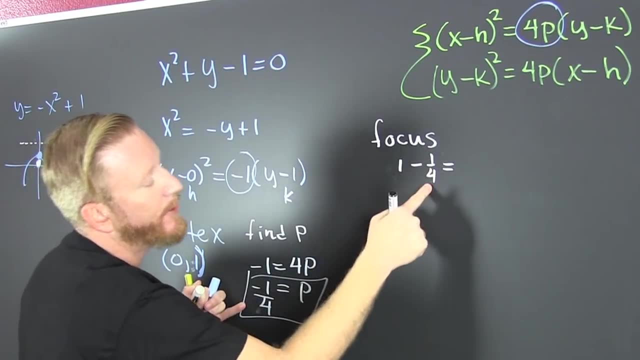 I take that y, 1, and I subtract off my 1 fourth, 1 fourth and that's wait for it, 1.. What is that? Zip zap zo, That's 3 fourths. So my focus is that's my new y. My x stays. 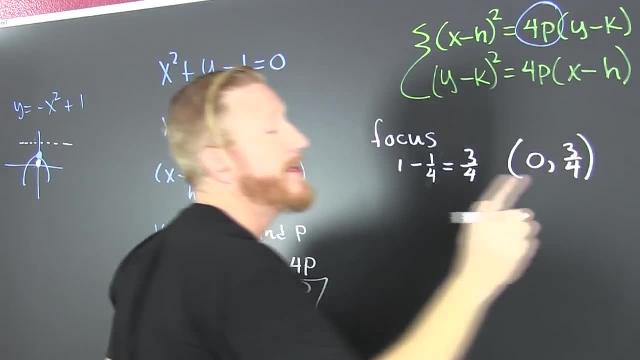 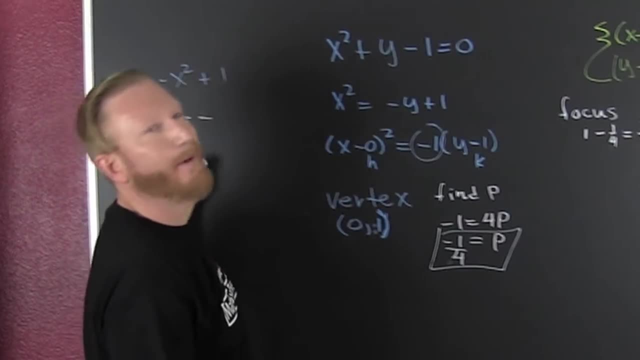 the same, It's still 0, 3 fourths. So if we were making a nice non-basic graph, that point there would be at 0, 3 fourths. I made a pick, So let's find the directrix, The directrix. 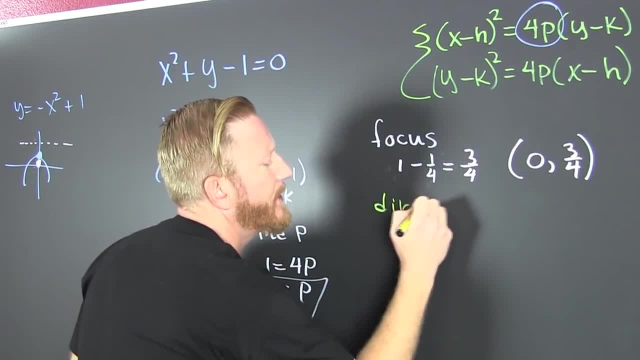 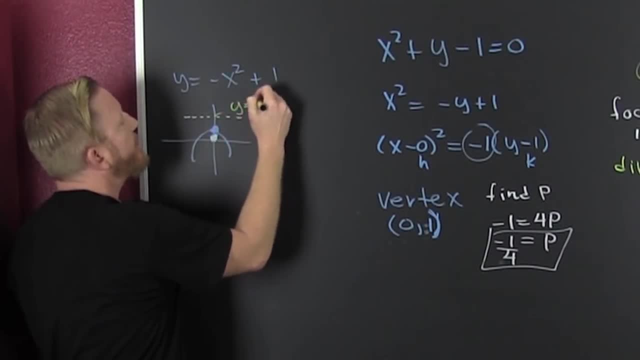 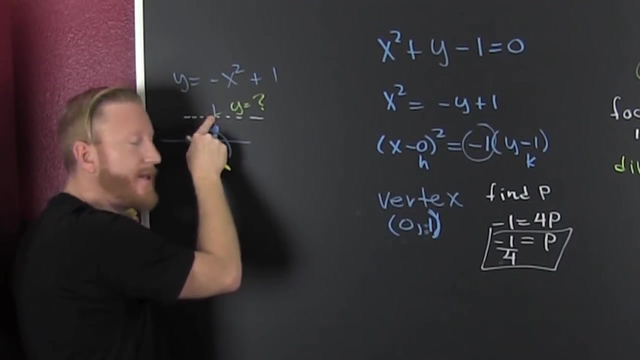 I direct your attention, The directrix, that's this line, Whose line? This line Y is equal to something? Is that bigger than or smaller than the vertex That's bigger than taller than higher than It's above? So I'm going to go and I'm going. 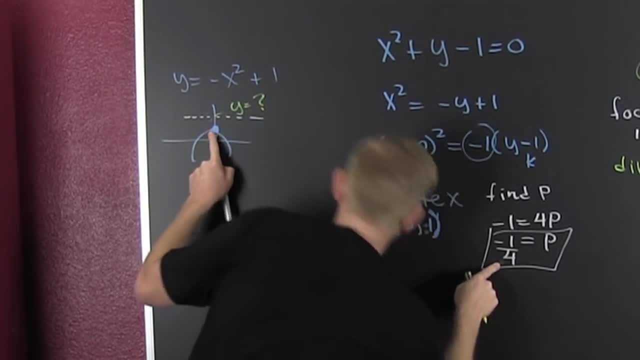 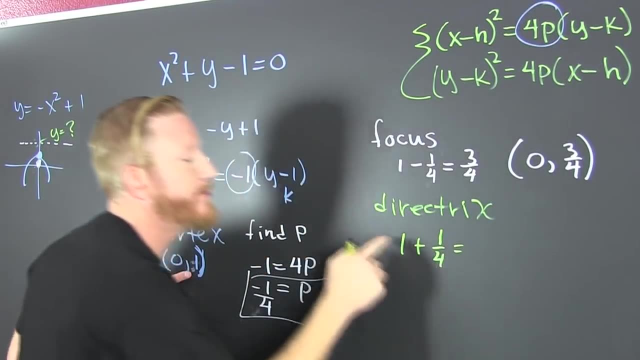 to add the 1 fourth to it. to what The y value? What's the y value? It's 1.. So then I'm going to take that 1 and I'm adding that 1 fourth to it, And when I do, zip, zap zo, Mr Emory. 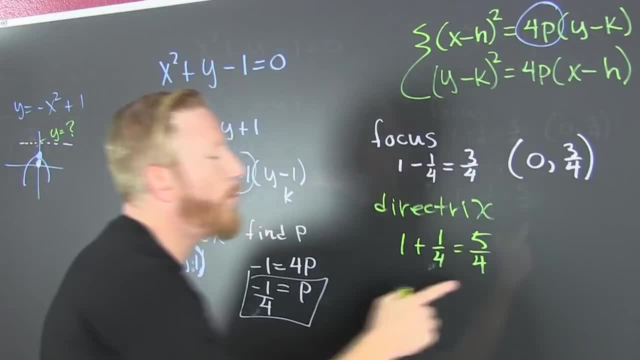 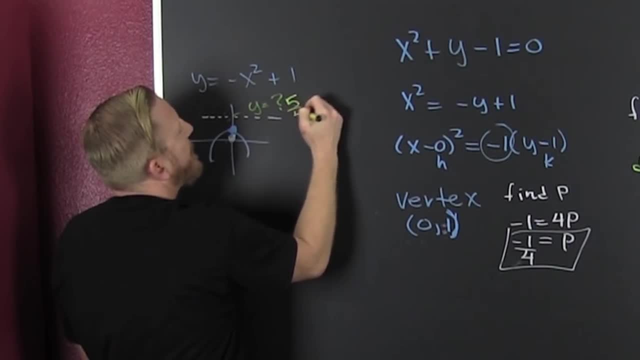 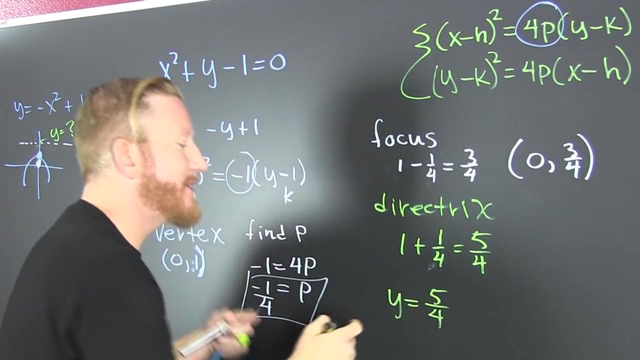 that's 5 fourths, For sure, for sure. So that's my new y, Which y, This guy Y was what Y was 5 fourths, And I'm going to write it down here: Y is equal to 5 fourths. So if I was going to properly draw this graph, it would look like this: 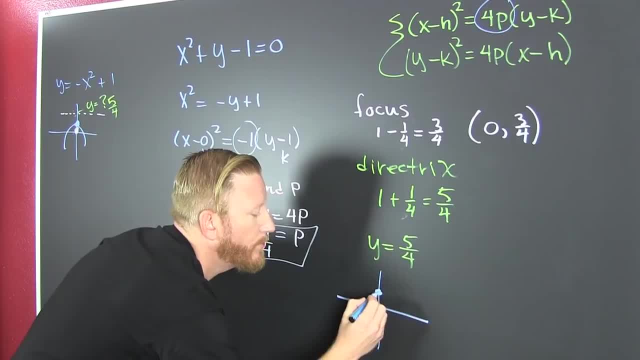 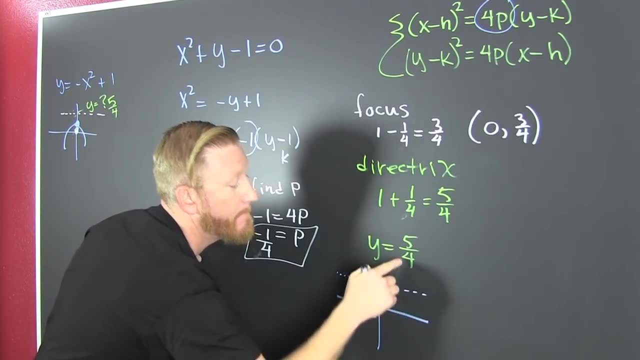 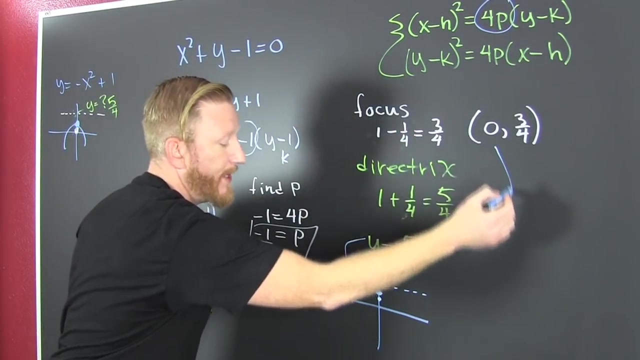 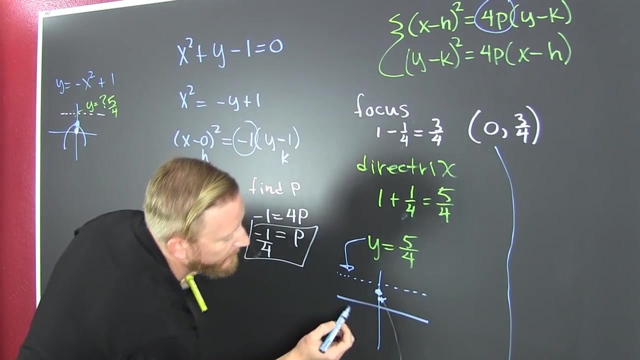 Boom O, What's that? That's my focus. What's this? My directrix? chiarito, Previous to number 4.. And then what's this? That's my focus. So then it's: all points equal distance from that dot and this guy. So this and that Those 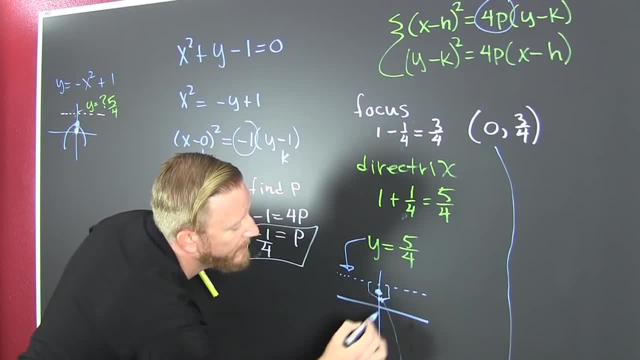 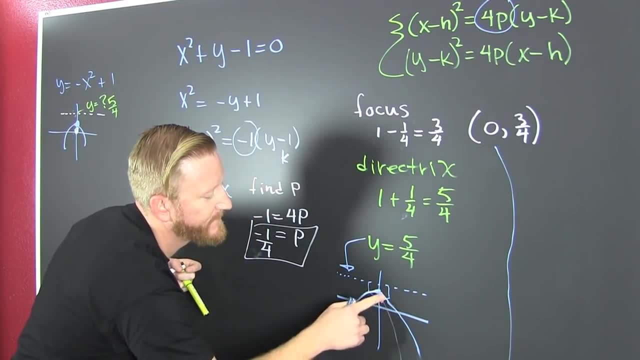 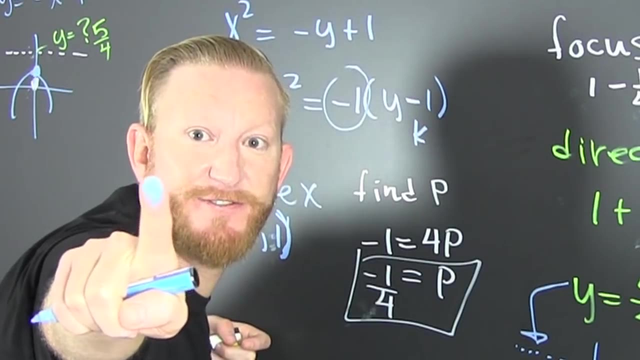 look equal and this and that. Does it look like somebody's jumping? Ah, no, almost Damn Ew. Ew. Does it look like I choked a Smurf? We're sorry. the number you have dialed is not in service at this time.